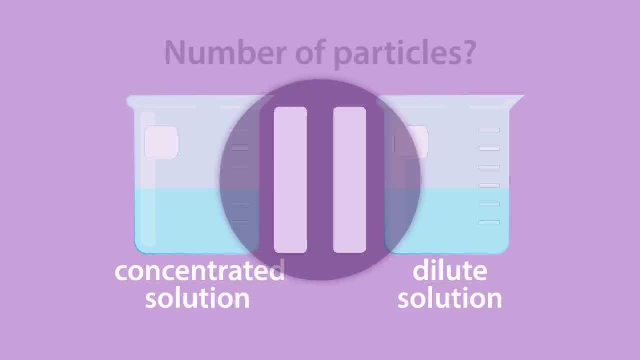 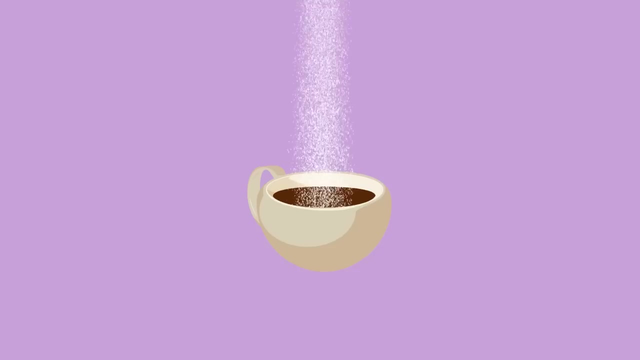 solution. Pause, think and continue when ready. The number of particles in a concentrated solution is greater than the number of particles found in a dilute solution. Think about when you sweeten a drink by adding sugar. The more sugar you add, the sweeter the drink tastes. We can calculate this using two-formulae and 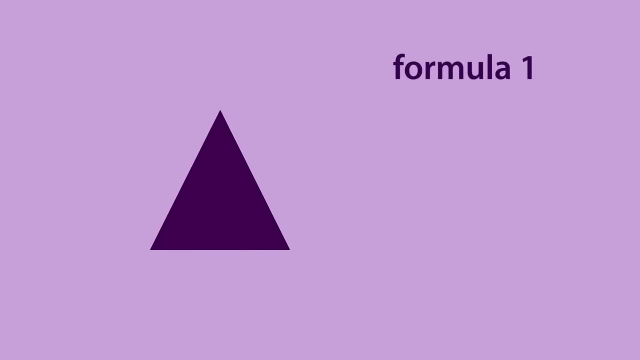 accompanying formula triangles. The first way of calculating concentration is to use moles, an amount of a chemical substance and divide it by its volume. Here's the formula triangle for this. Most of the time volumes are measured in cubic centimetres, so 1000. 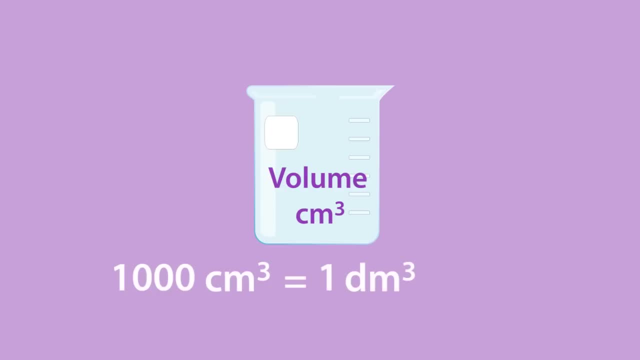 cubic centimetres is equal to 1 decimetre cubed or 1 litre. So how many decimetre cubed is 500 cubic centimetres? Pause, think and continue when ready To get the answer. you need to divide 500 cubic centimetres by 1000, so 500 cubic centimetres. 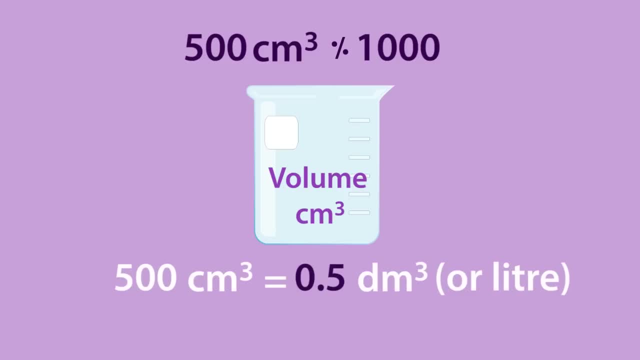 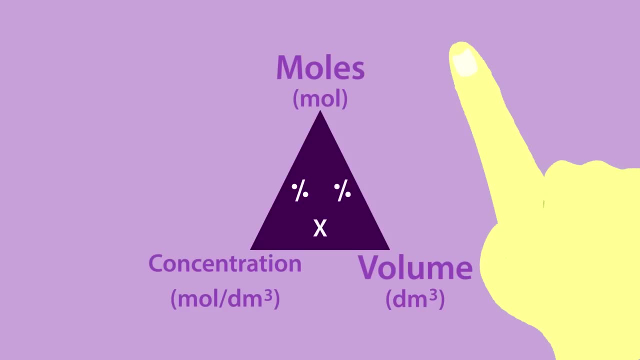 is the same as 0.5 decimetre cubed. Did you get it right? You can find any of these quantities by covering up the one you're looking for with your finger. For example, if you cover moles, you can find this by multiplying the concentration by the. 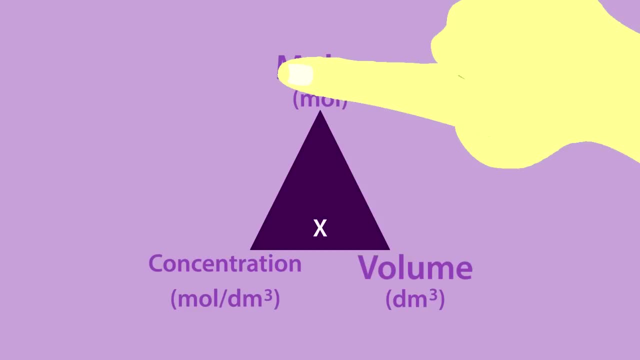 volume. This is because any two terms on the bottom of a formula triangle are always multiplied together. If you want to find the concentration, you cover this and divide the number of moles by the volume. Let's try this now. If you have 2 moles of salt and 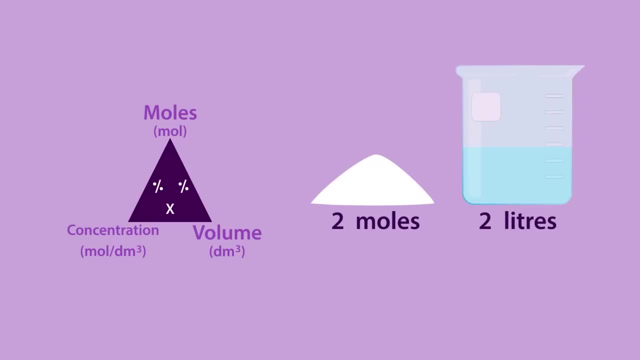 dissolve it in 2 litres of water. use the formula triangle to calculate the concentration of the salt solution. Don't forget the units. Pause, write down you're working out and continue when ready. 2 moles divided by 2 litres is equal to 1 mole per decimetre cubed. Did you get it? 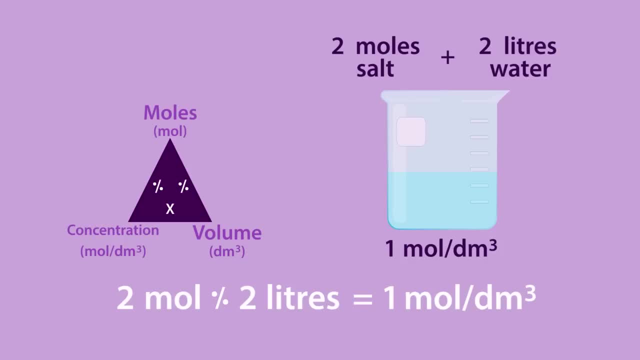 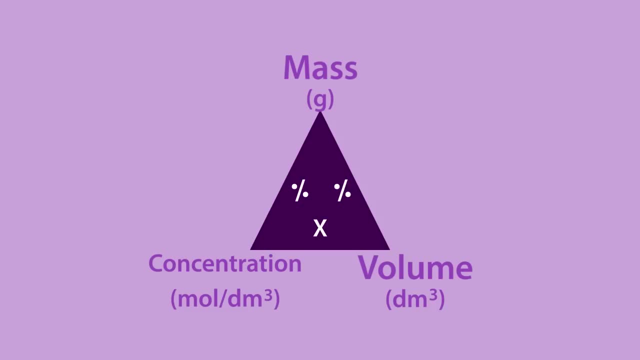 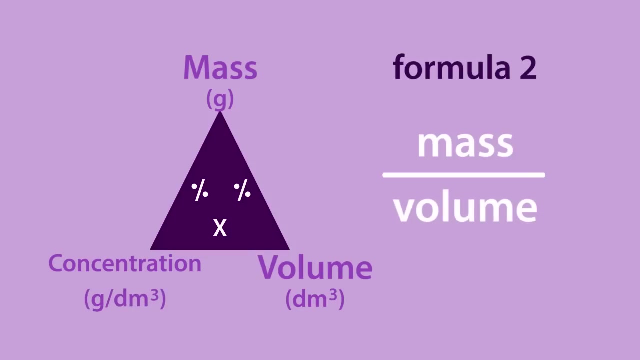 right, And did you include your units? The second way of calculating the concentration is very similar, except sometimes we use a mass of a substance divided by volume rather than a mole of a substance. The formula is mass divided by volume and has the unit grams per decimetre cubed rather than moles per. 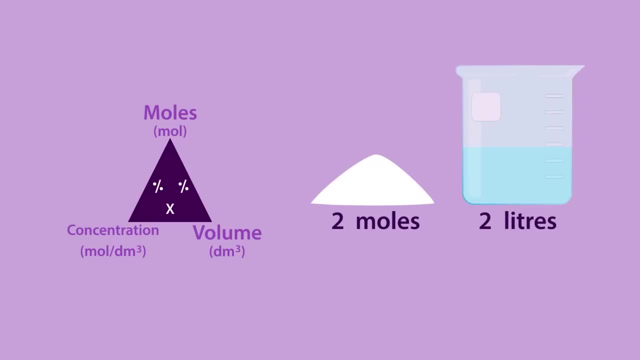 dissolve it in 2 litres of water. use the formula triangle to calculate the concentration of the salt solution. Don't forget the units. Pause, write down you're working out and continue when ready. 2 moles divided by 2 litres is equal to 1 mole per decimetre cubed. Did you get it? 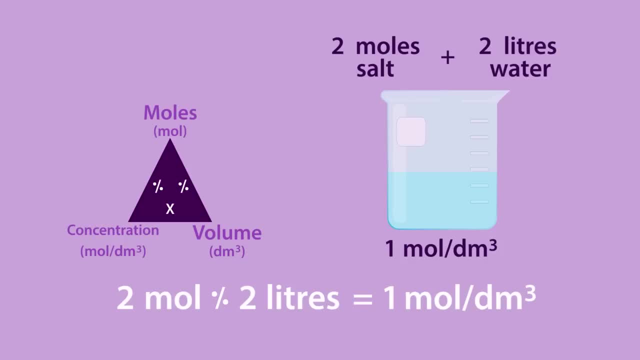 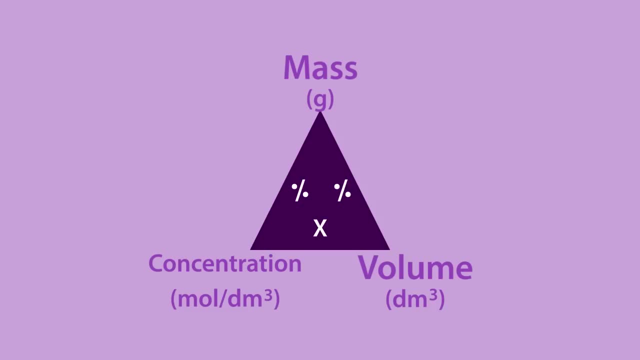 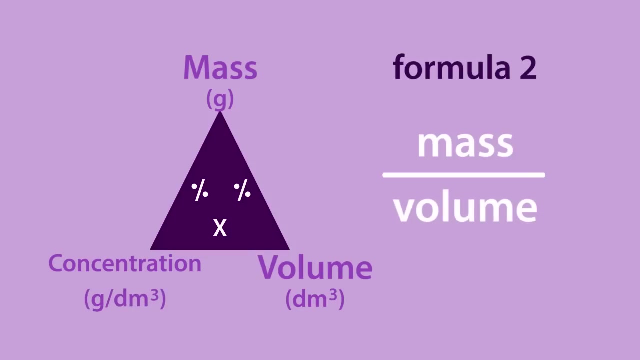 right, And did you include your units? The second way of calculating the concentration is very similar, except sometimes we use a mass of a substance divided by volume rather than a mole of a substance. The formula is mass divided by volume and has the unit grams per decimetre cubed rather than moles per. 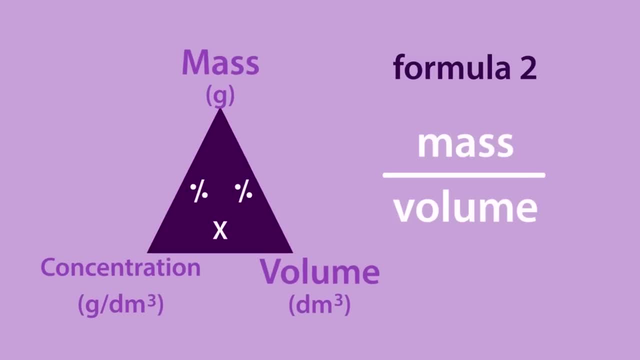 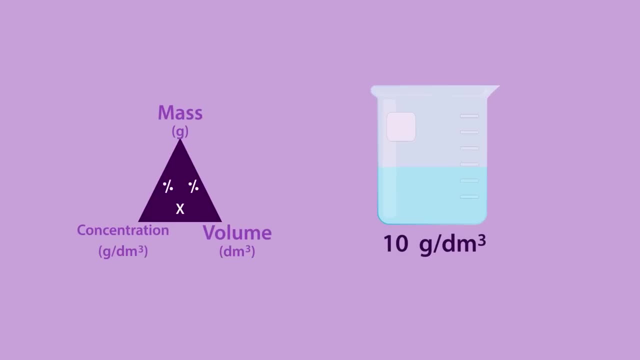 decimetre cubed. It's formula triangle looks like this. Let's try a challenge If you know that you need a 10g per decimetre cubed salt solution and have to dissolve it to a volume of 250ccm. 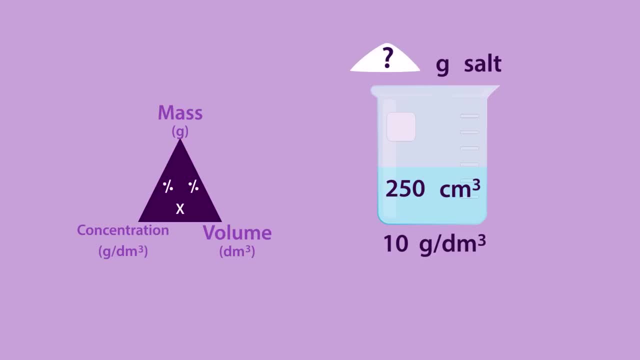 what mass of salt will you need to dissolve? Pause and write down your working out. Don't forget that you have to convert the volume from cubic centimetres to decimetre cubed. Continue when ready. 2 moles divided by 2 litres is equal to 1 mole per decimetre cubed. 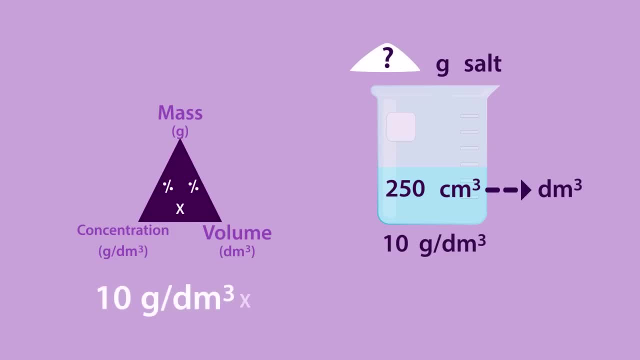 2 moles divided by 2 litres is equal to 1 mole per decimetre cubed. Continue when ready. 2 moles divided by 2 litres is equal to 1 mole per decimetre cubed. Press and hold the fever stop button when the temperature drops below 60°F based. 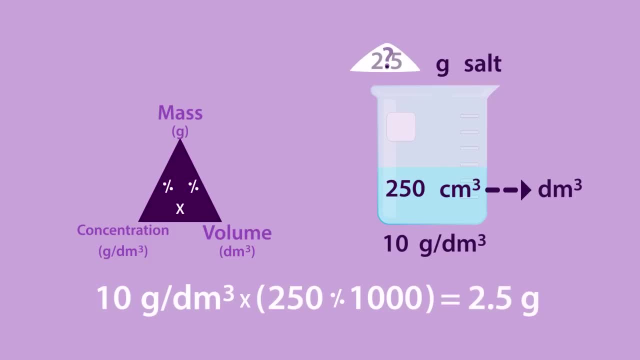 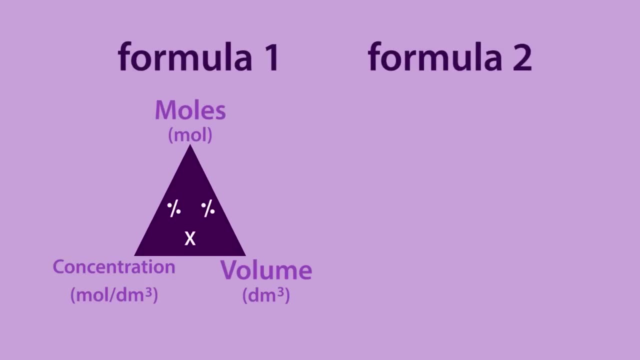 on the distance added to the solar lighter and repeat the procedure. 1 mole per decimetre cubed will be the total mass of a product by the variable warm to write it down. If there is a strong temperature, the finished product can keep cooling for up to 30 minutes. 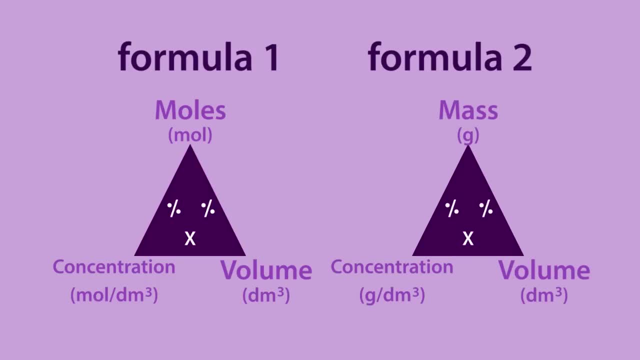 and make a lot of produce in a day, so we will just let the temperature drop, Get ready Welding When the formula is solid. this also means that we have massive milk, So give this an abundance of cream. A steel mould will weigh half the size of a figure using 163.. pracryl, Now that it's 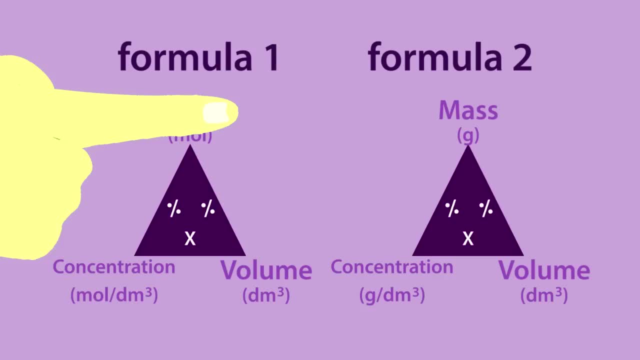 soldered to the nationally market. it's William作 relaxation تعampilsthis月 ag commission divided by carbon offerings or division as shown in the triangle.